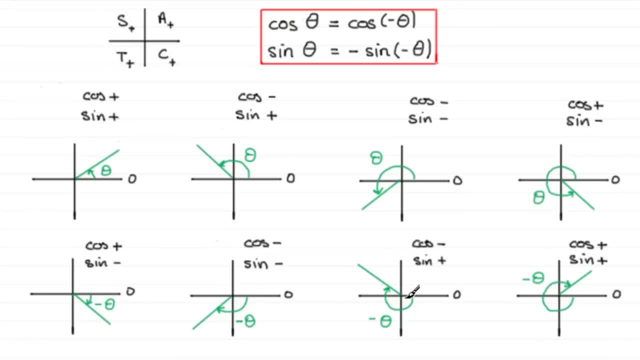 two diagrams. I've taken reflex angles and you can see I've drawn the negative counterpart. okay, for each of the ones above. So when it comes to taking the cosine, say, of an acute angle, here, the cosine of any acute angle would be in the quadrant and its trig ratio will be positive. cosine will always return a. 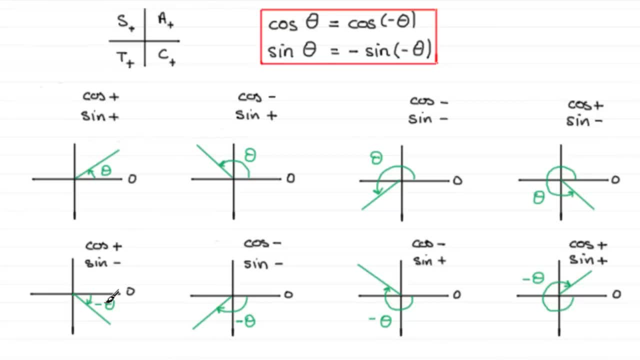 positive value. when you do the cosine of a negative angle, you'll get exactly the same value, because cosine in the fourth quadrant is always positive. so you can see we get exactly the same value. but when it comes to taking the sine of this acute angle, in the first quadrant is positive but in the fourth quadrant the 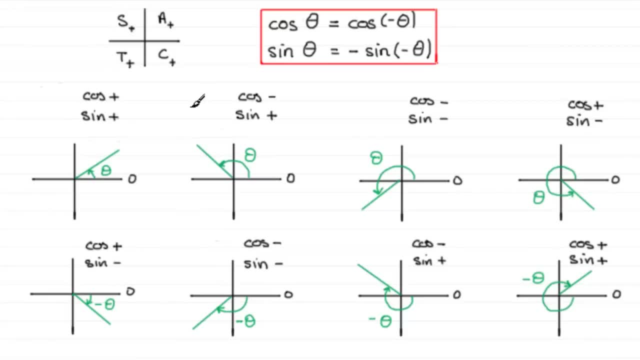 sine of a negative angle is negative. only cosine is positive. so in order for these two to be the same, for taking the sine, we have to negate this answer. so if we do, sine of this angle is equal to minus the sine of this angle down here, And the same kind of argument is true for each of these diagrams. You might. 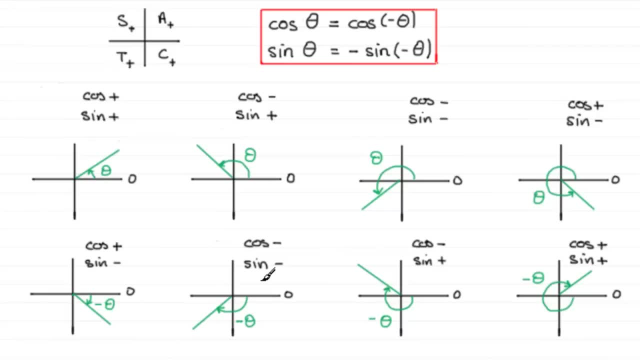 want to just work your way through them, But essentially for this one here, this obtuse angle, cosine would be negative for it in the second quadrant because only sine is positive. But when you take the negative angle, can you see? it puts us in the third quadrant and 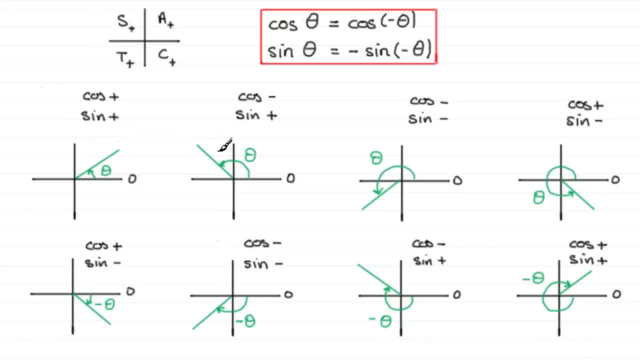 cosine is negative in this quadrant. So cosine is negative in both this quadrant and this quadrant, So they would still be equal to one another. The cosine of theta is equal to the cosine of minus theta, But when it comes to the sine, the sine of this angle- 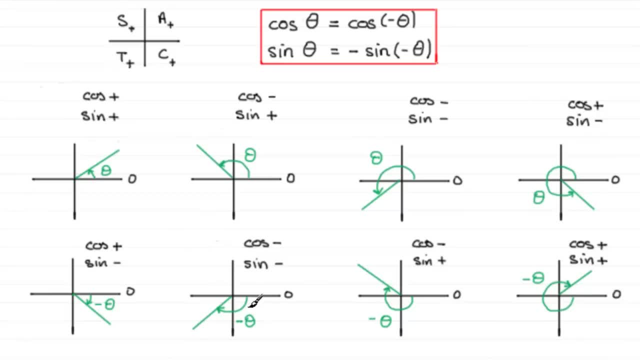 in the second quadrant is positive. But when we take the sine of the negative angle here in the third quadrant, here, because tan is the only one that's positive, we take the cosine of the negative angle here in the third quadrant, and cosine is the only one that's.